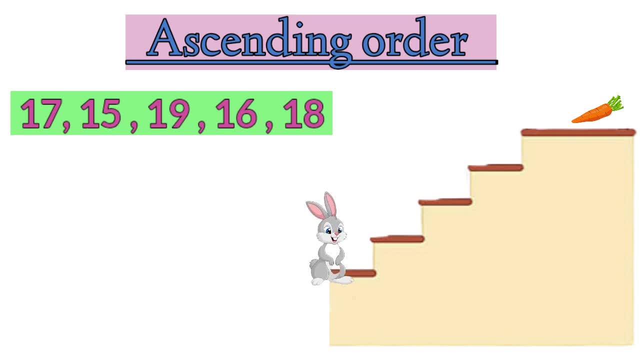 So the smallest number is number 15.. Then comes number 16.. Next is number 17.. Followed by number 18.. And lastly number 19.. So finally, Mr Pony got his carrot. Among all the numbers, number 19 is the greatest number And number 15 is the 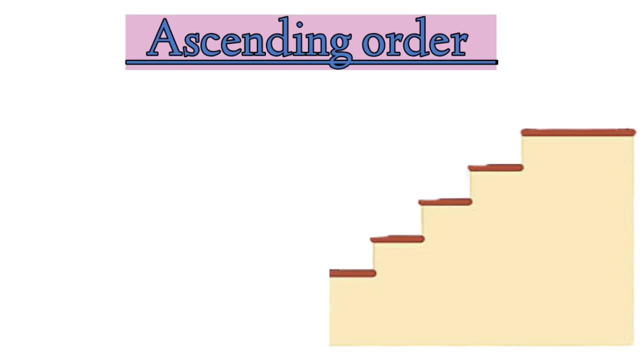 greatest number. So the smallest number is number 15.. So the smallest number is number smallest number. Now let's arrange another group of numbers in ascending order. The numbers are 32,, 31,, 29,, 33, 30. Children- let's help Mr Pony once again to get his carrot. 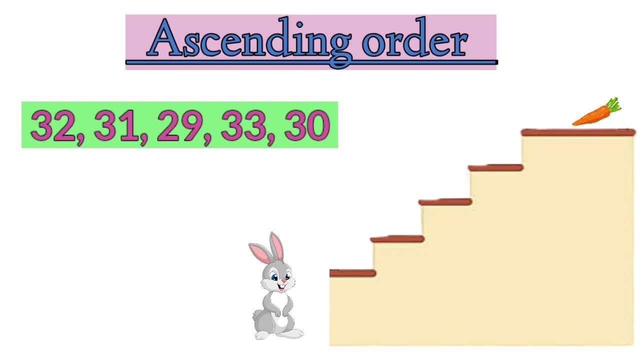 by arranging the numbers in ascending order. Among these given numbers, which number do you think is the smallest number? That's right. number 29 is the smallest number And it will come in the first place. Next will be number 30. Then comes number 31. Followed by 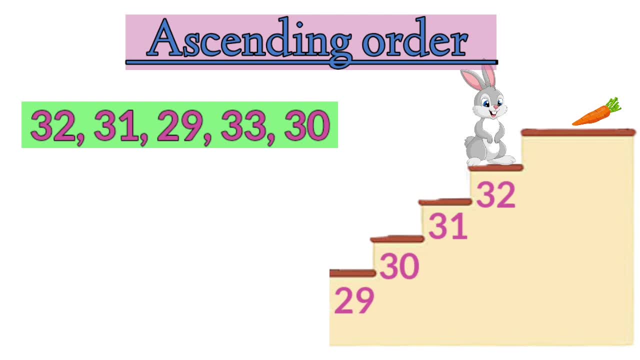 number 32.. And lastly, number 33.. Children, finally, with your help, Mr Pony got his yummy carrot Among these numbers, which is the smallest number? Yes, number 29 is the smallest number And which is the greatest number? Very good, Number 33 is the greatest number. Remember that in ascending order. 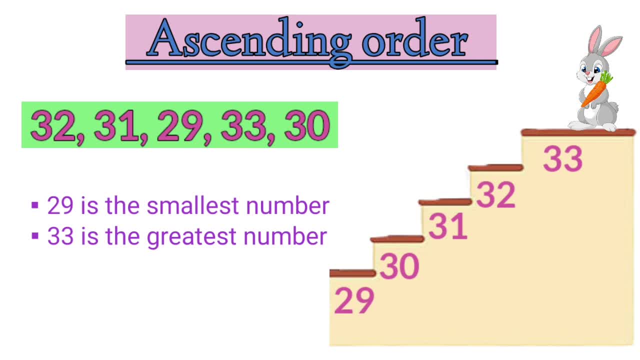 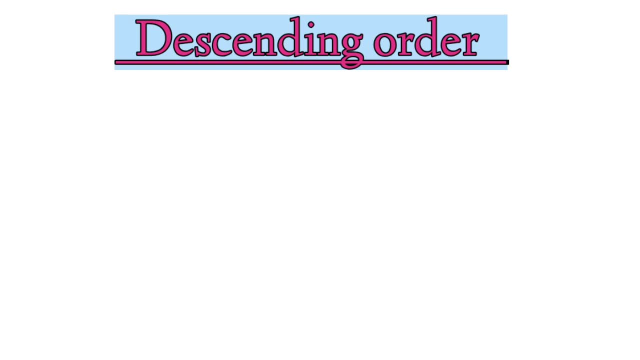 we should always start with the smallest number and end with the greatest number. Descending order. Descending order means arranging numbers from big to small, Or when we move from upstairs to downstairs. it is called descending order. Always remember that in descending order. 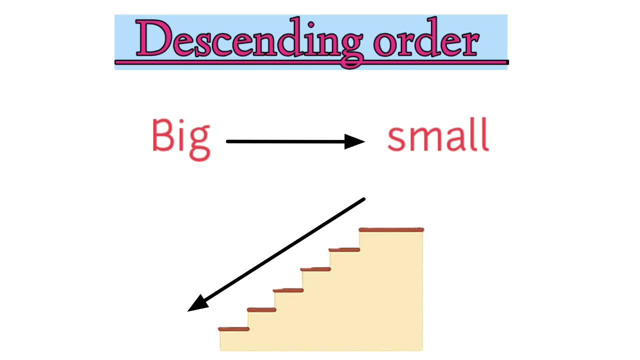 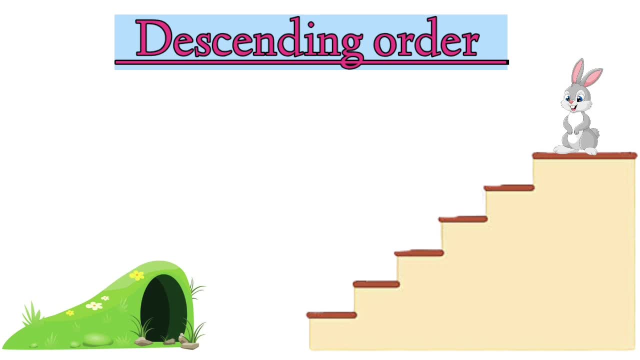 the number always keep on decreasing. All right Now children, after eating the carrot, wants to go down to get back home, But for that we need to help him get down by arranging the numbers in descending order. So let's all help him to get down from the stairs by arranging the 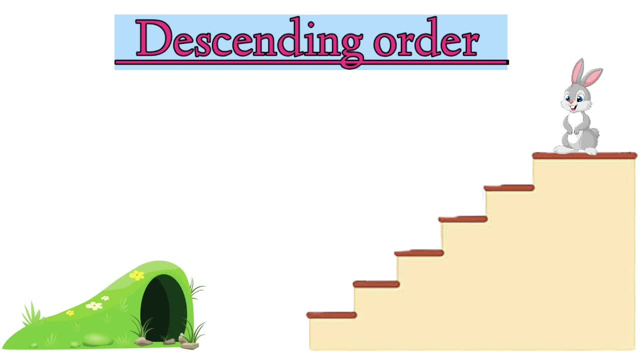 given numbers in descending order. All right, The numbers are 47,, 45,, 43,, 46,, 44.. Children: which number do you think will come on top? Yes, the greatest number will come on top right. So the 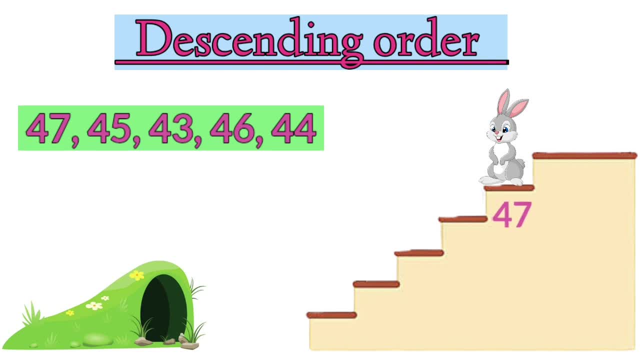 greatest number is number 47.. Next number will be number 46. Then comes number 45, followed by number 44. And finally the smallest number, that is number 43. Therefore, Mr Punny finally gets down to go back to his home Children. let's do one more example by. 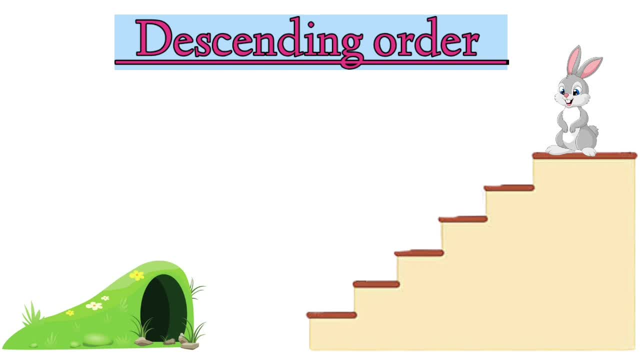 arranging the numbers in descending order and help Mr Punny to get back to his home. We have number 11, 9,, 12,, 8,, 10.. Now let's all arrange them in descending order: Children, which is the. 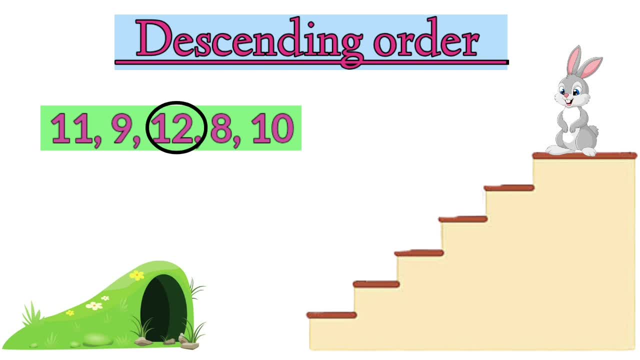 greatest number. Yes, number 12 is the greatest number. So number 12 will come on the top. Next number will be number 11.. Then comes number 10, followed by number 9.. And the smallest number, that is number 8, will come at the bottom. So, children, that's how Mr Punny reaches his home: by arranging 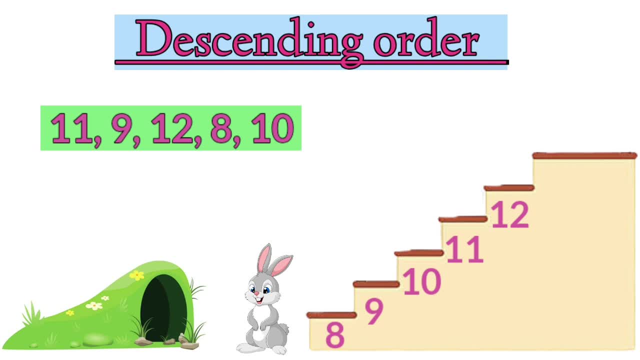 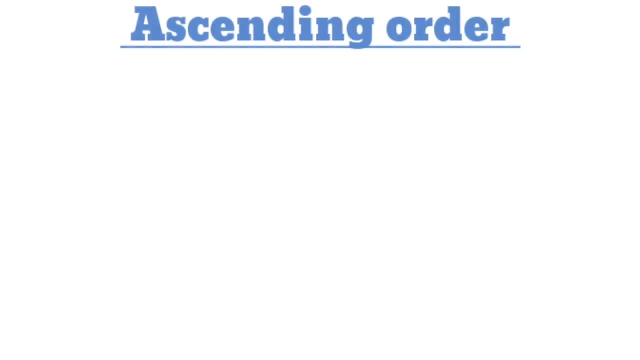 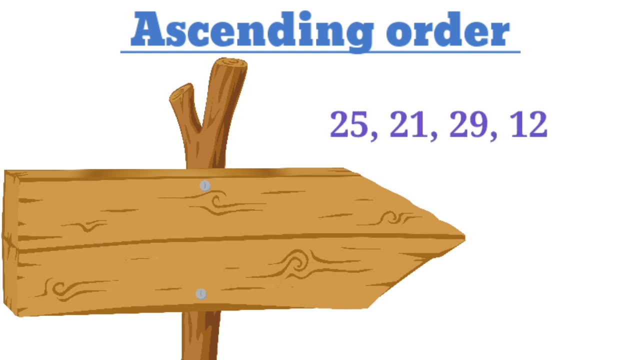 numbers in descending order. So, children, let's all arrange them in descending order, And the smallest descending order. now let's do a quick review. first let's arrange the numbers in ascending order. we have 25, 21, 29, 12, 15 children among the given numbers. 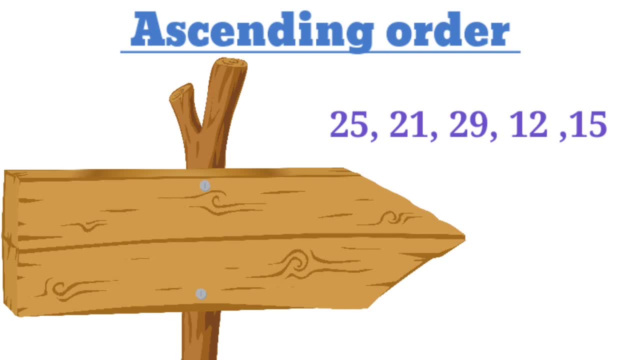 which is the smallest number. very good, number 12 is the smallest number and which is the greatest number. that's right. number 29 is the greatest number. in ascending order, we should start with the smallest number. so the smallest number, that is, number 12, will come first. next number will be number 15, then comes